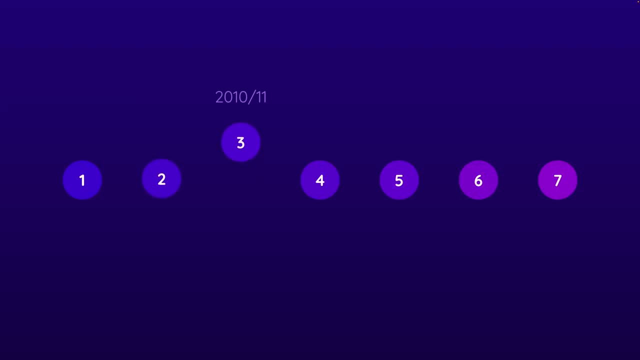 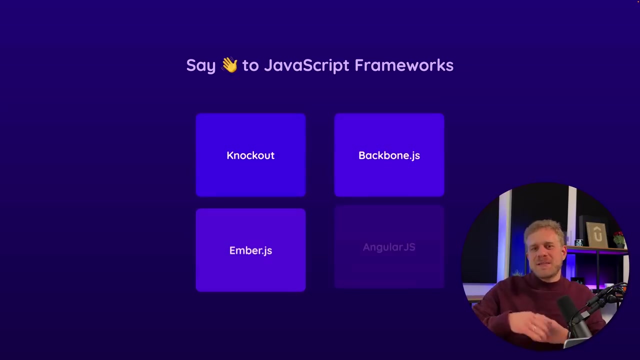 jQuery quickly reached its limits. It was around 2010-11 that we entered the third phase of JavaScript framework evolution, if you want to call it like that, With the introduction of Emberjs, Backbonejs, Knockoutjs and, most importantly, Angularjs- Angular 1,. 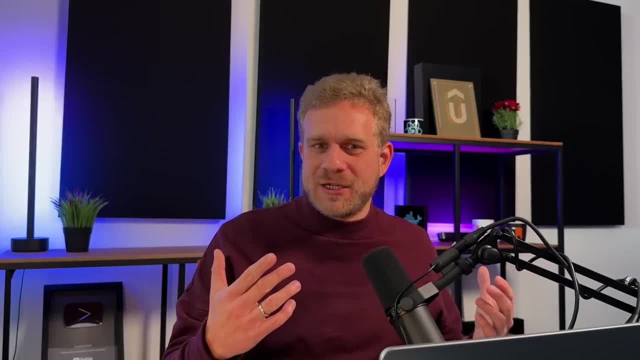 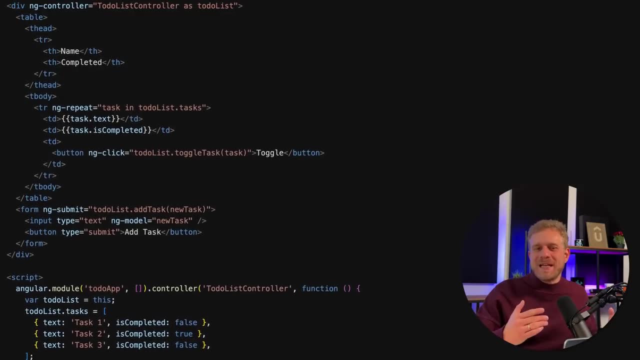 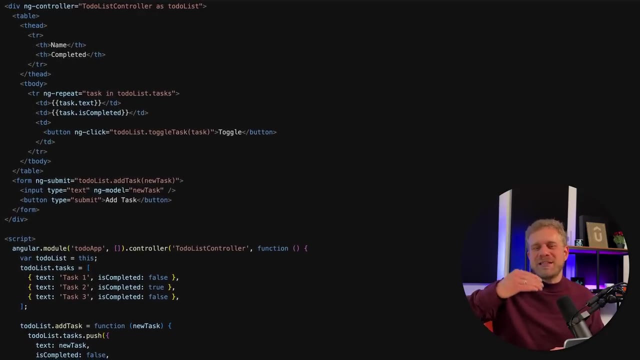 we got some powerful frameworks that made it much easier to build complex web user interfaces that were powered by client-side JavaScript. These frameworks helped with state management. they made it much easier to reflect state changes back into the HTML document, so that you didn't have to write every step on your own, as you did with jQuery. but of course, as always, it was not. 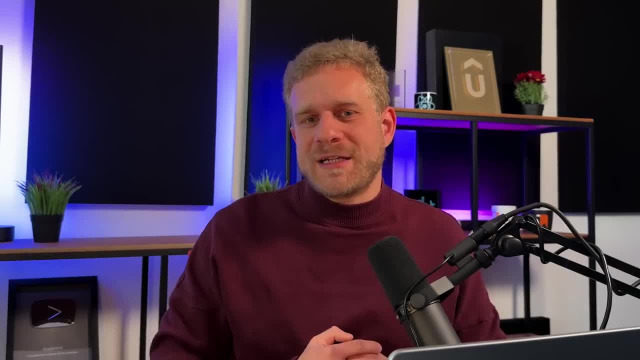 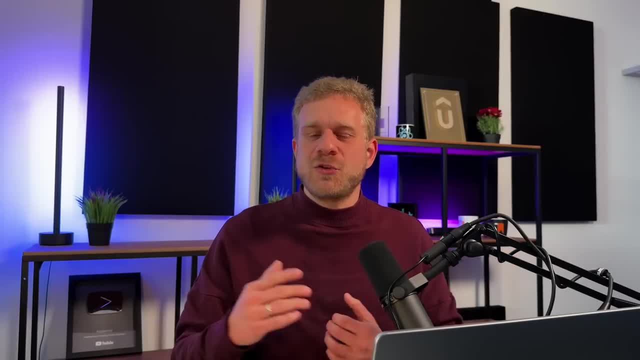 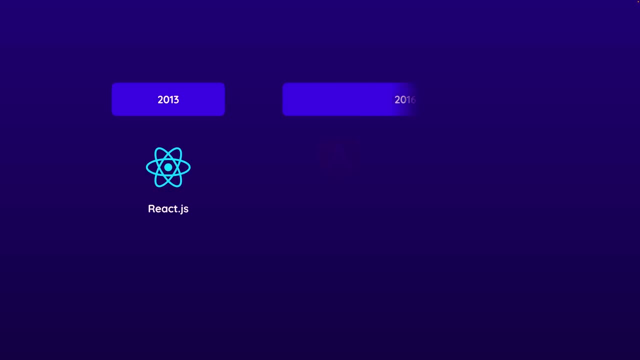 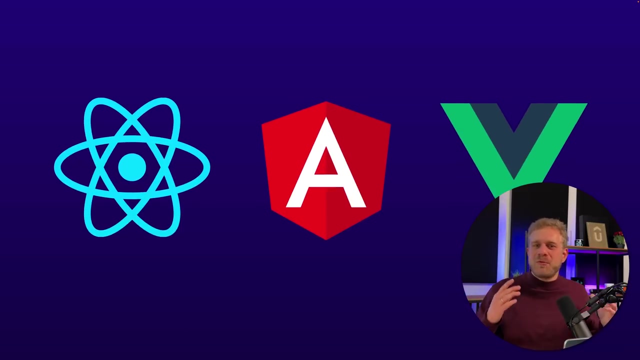 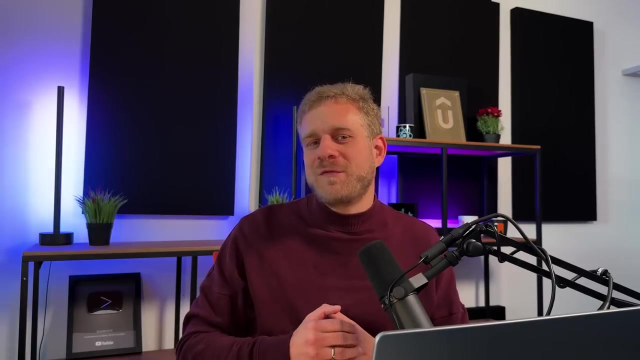 with today's React, but we got React in 2013, and in 2016 we got Angular and also Vuejs too, And these three frameworks are still the most important front-end JavaScript frameworks we can use today. Almost all more complex, modern JavaScript-driven web user interfaces are 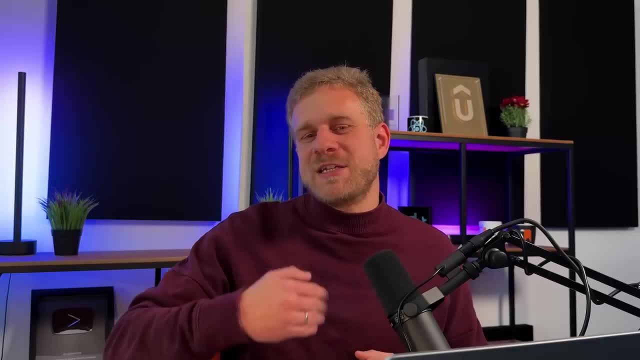 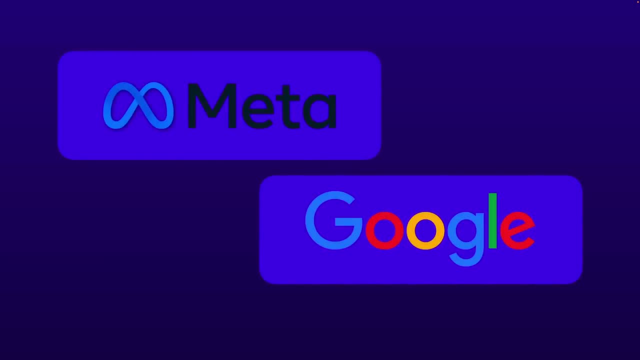 powered by one of these three frameworks. These three frameworks are still the most important front-end JavaScript frameworks, and that's why we definitely entered a new evolution phase with the introduction of these frameworks. Of course, part of the reason why we still use React and Angular is that those are backed by Facebook or Meta in case of React and Google in case of. 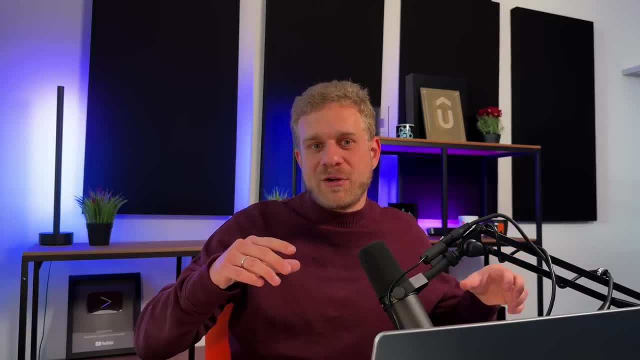 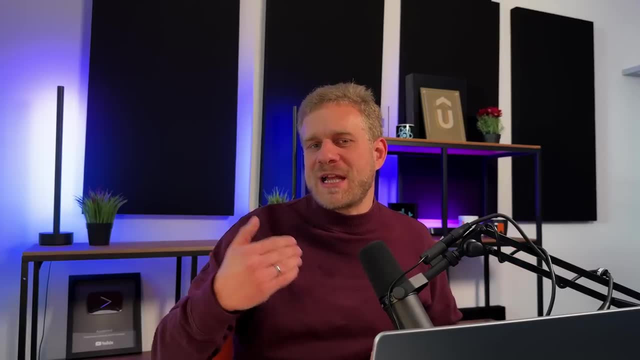 Angular. So naturally, there are big companies using these frameworks because they developed them themselves, And that, of course, helped with making sure that these frameworks sticked around and did not get replaced by new frameworks, but instead evolved themselves. As I mentioned, the React you know today and the React you don't know today are not the same thing. The React you know. 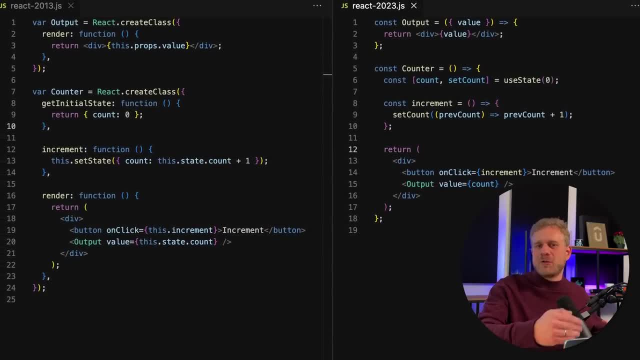 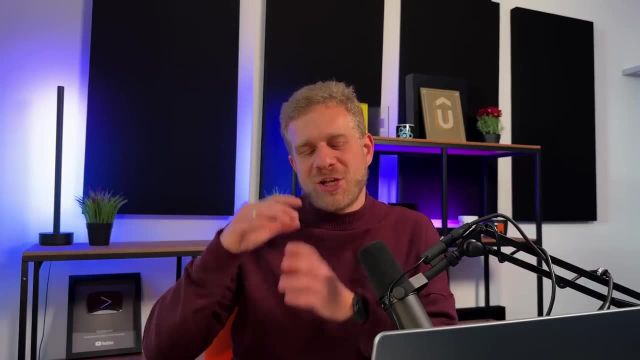 right today doesn't have that much to do with the React code you wrote back then in 2013.. Nonetheless, you could say that we then entered another evolutionary phase, because we did not just have these frameworks, but we got lots of JavaScript frameworks. At some point, you could 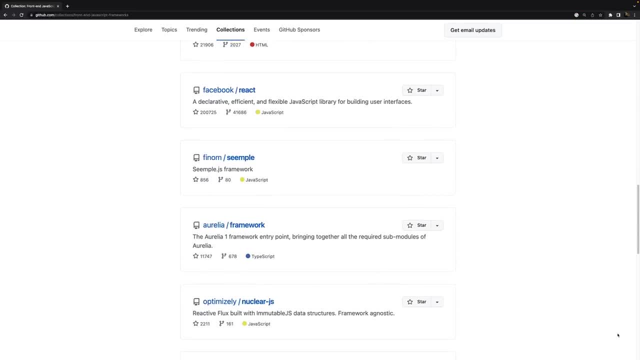 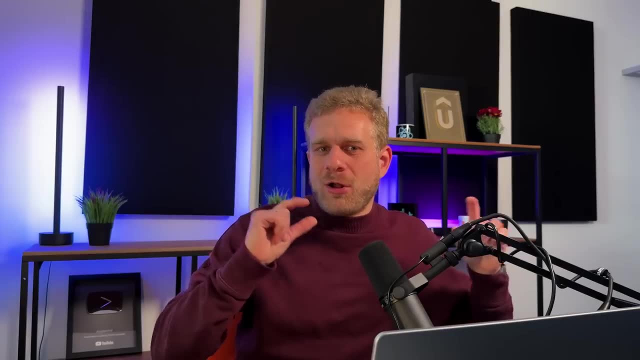 think that a new JavaScript framework was coming out every day. Now, to be honest, most of these frameworks are just niche frameworks. If you want to get a job, you're way better off learning React or Angular. They all solve different problems in different ways, and together they were. 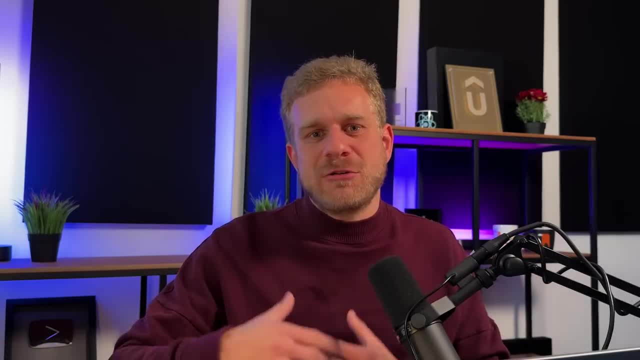 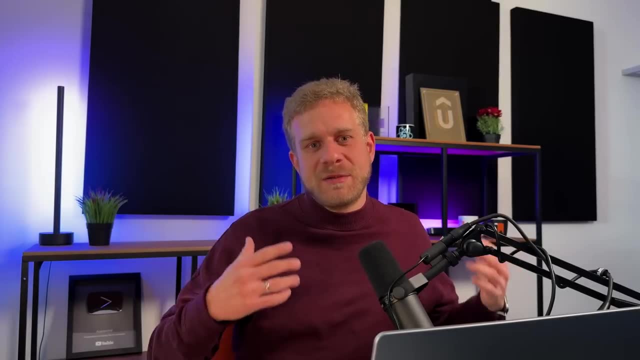 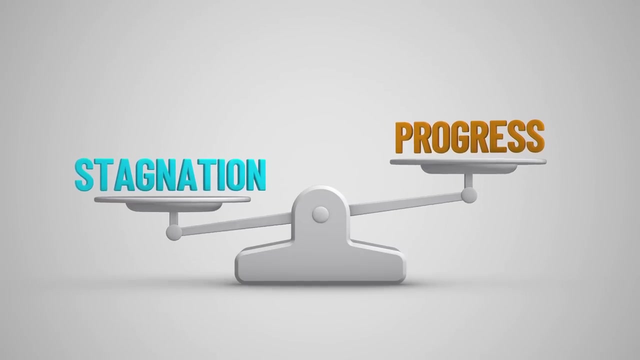 super important because they also pushed React and Angular and Vue forward, because those also had to reinvent themselves over time, as mentioned before, because otherwise they would simply have been overtaken. So this entire phase of continuous improvement of these frameworks, of the addition of new features and so on, was another super important phase in the history of frontend JavaScript. 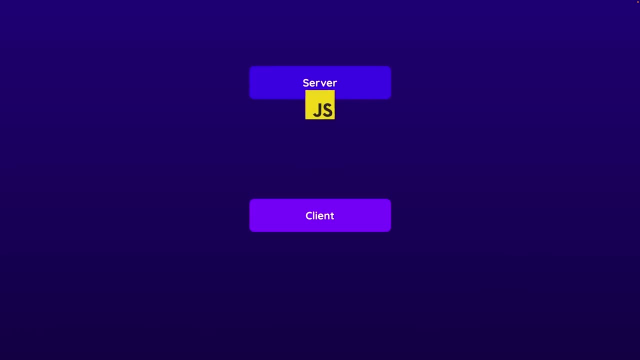 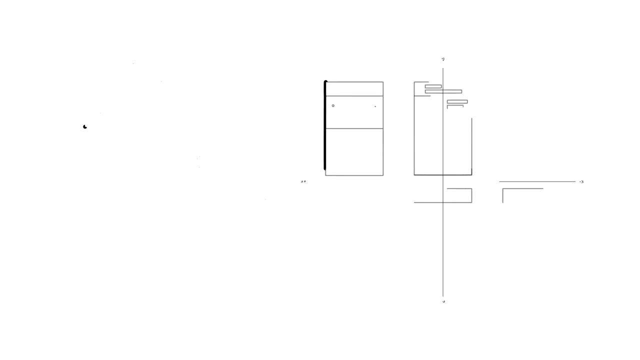 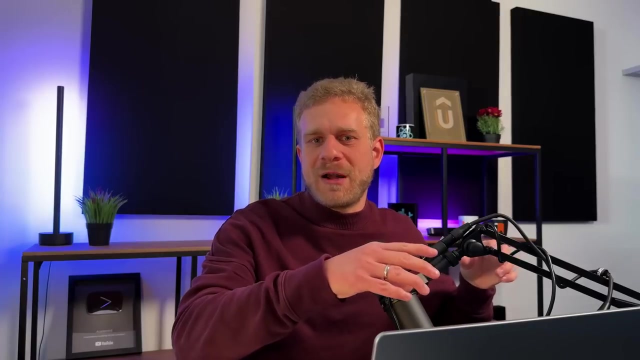 development. Now, all these frameworks came up because we wanted to put more and more JavaScript code into the browser. We wanted to control the entire interface for the entire server from inside the browser, because that allowed us to build highly interactive user experiences. But the problem with that approach is that more and more JavaScript code moved into the browser. 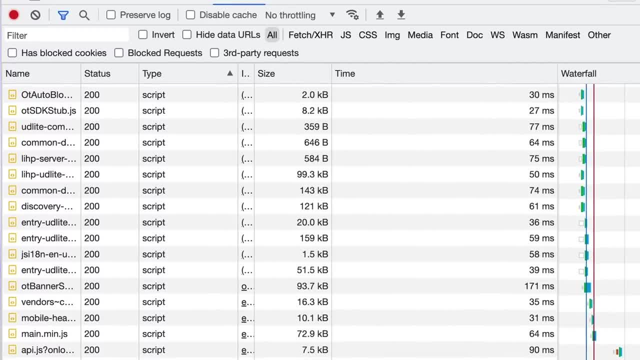 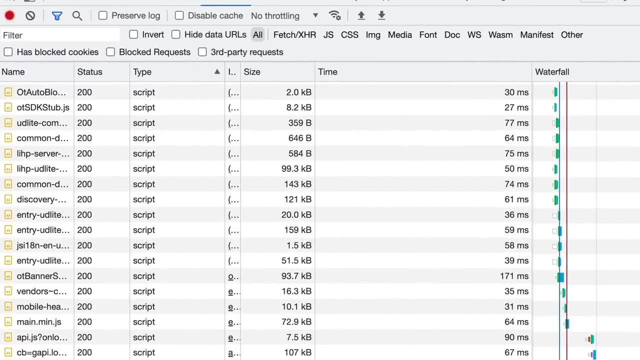 away from the server, away from the backend. Now, as a result, on many web pages that use these frameworks, users have to download a lot of JavaScript code before the website becomes interactive, which can be a problem if you have a slow internet connection. In addition, since everything happens in, the browser. data must be fetched and sent all the time and for all these reasons, we might have pushed too far. having everything on the client side might not be perfect, and that's why we entered another phase of JavaScript frameworks. We moved towards static site generation and moving more logic away. 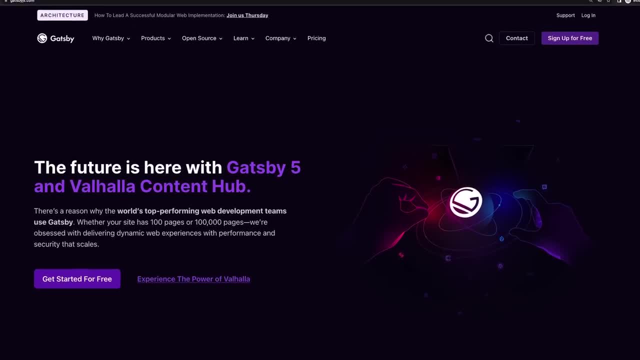 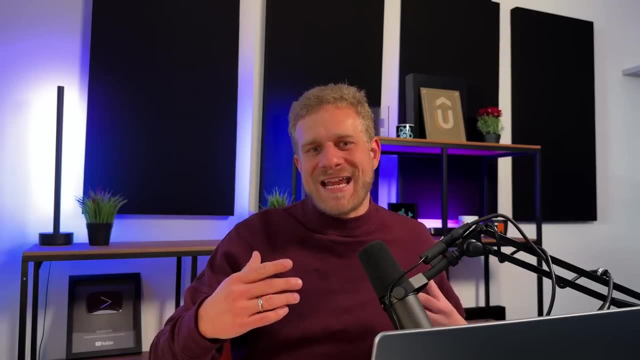 from the client side again. For example, with Gatsby and also Nextjs, we got solutions that allowed us to run some code on the server or even at build time, so that we could ship static apps which users could then visit, so that there was less client-side JavaScript code needed and less data fetching going. 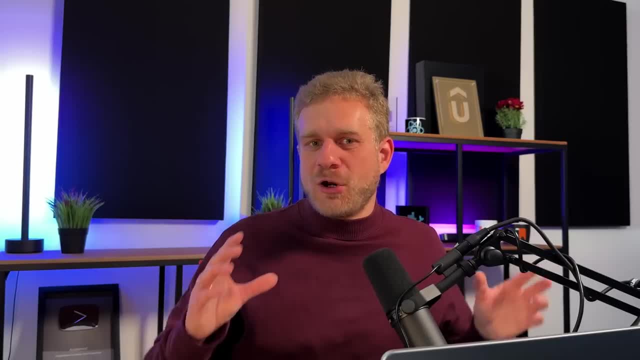 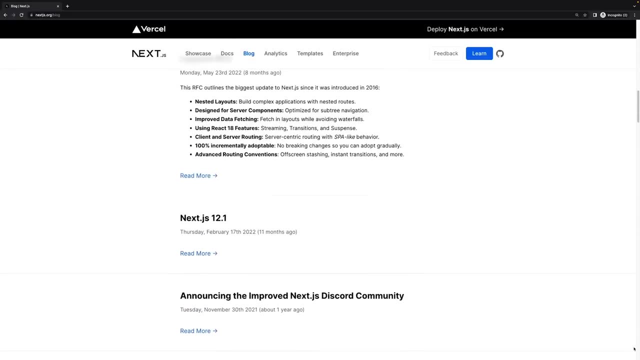 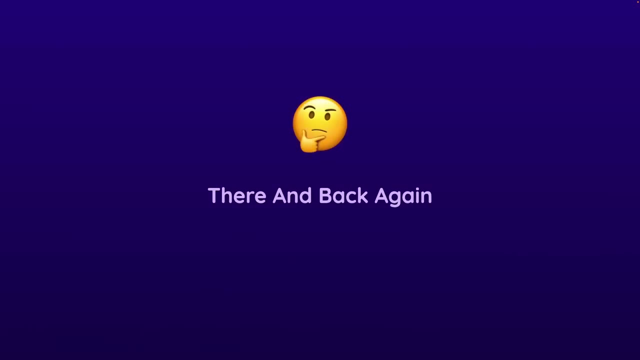 on when a user visits a website. Now, this phase, of course, isn't over- static site generation is still important, and Nextjs, for example, is still important- but also because it also continued to evolve. And that brings me to the last phase we entered up to this point, The phase where we are moving back. 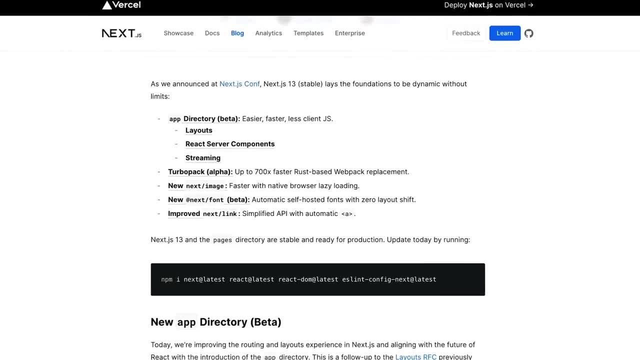 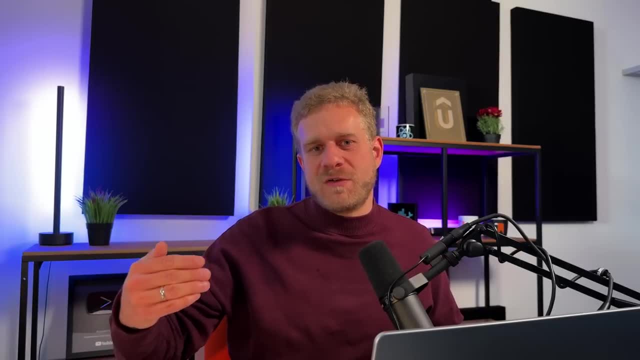 to full stack development With Nextjs 13. the Nextjs team, for example, introduced a brand new way of building Nextjs apps where way more work would happen on the server, where react server components would be able to run on the server instead of running on the server itself. So we 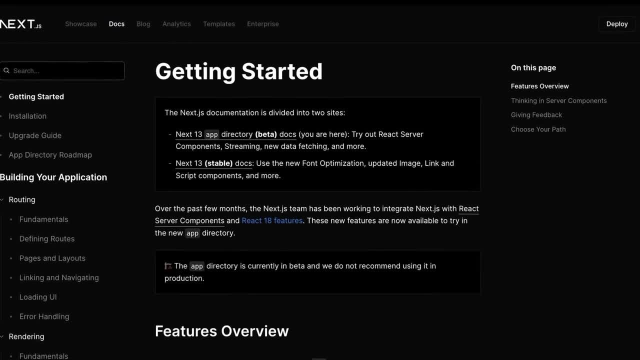 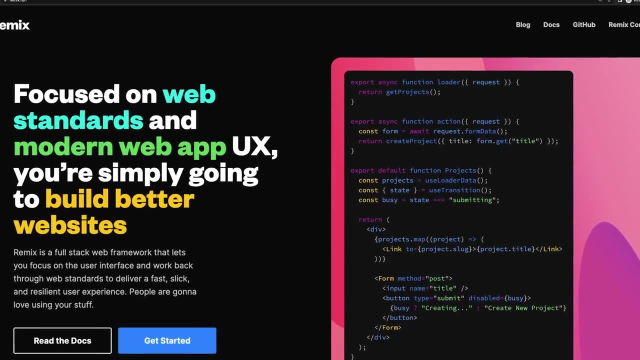 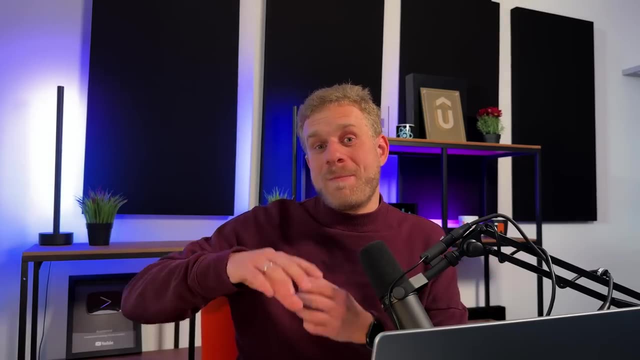 would be able to do more work on the server And even though this new feature is not finished and stable yet in Nextjs 13, it's definitely the future of Nextjs And we also have alternatives like Remix or Astro or Solid Start for Solidjs, which also move more work back to the server. 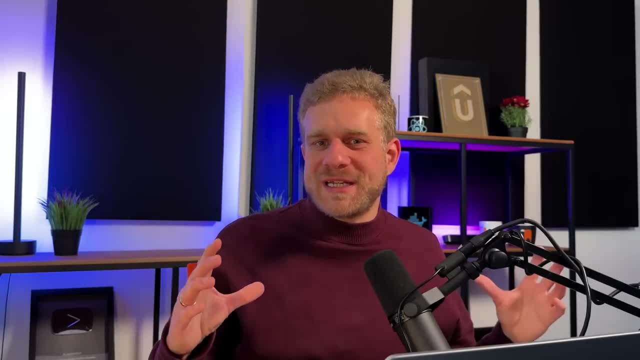 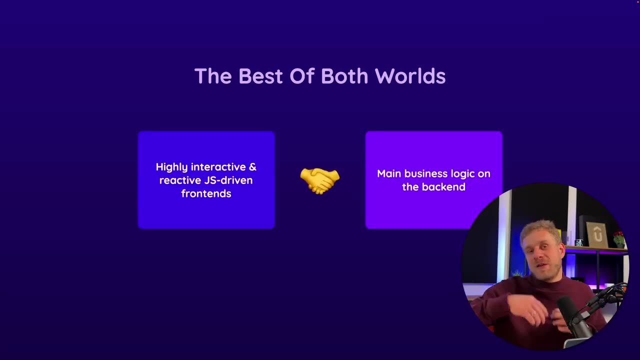 and which, ultimately, are about building complex, full stack applications which combine the best of both worlds, Allowing us to build highly interactive frontends, but with all the work done on the backend. that should best be done on the backend And in my opinion, this is definitely. 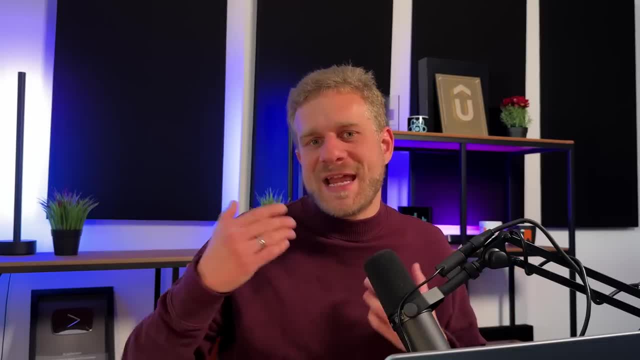 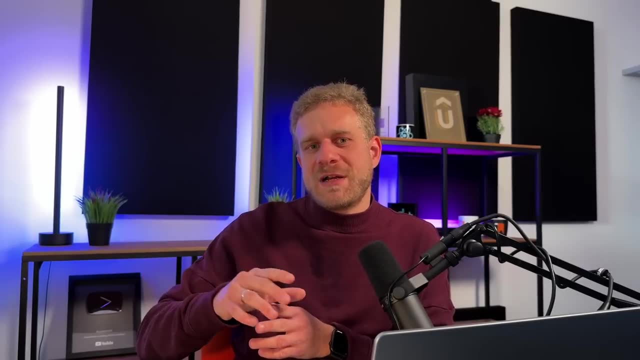 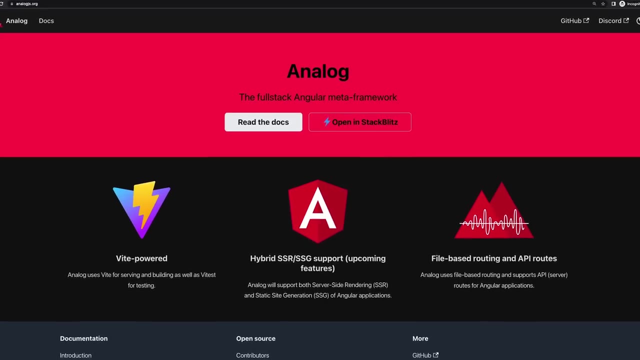 the way forward. We will still use React because ultimately, Next and Remix and so on still use React, But we will combine it with those meta frameworks to do more work on the server as well and to get the best of both worlds. Vue has Nextjs, Angular has Analogjs and, in my opinion, this trend. 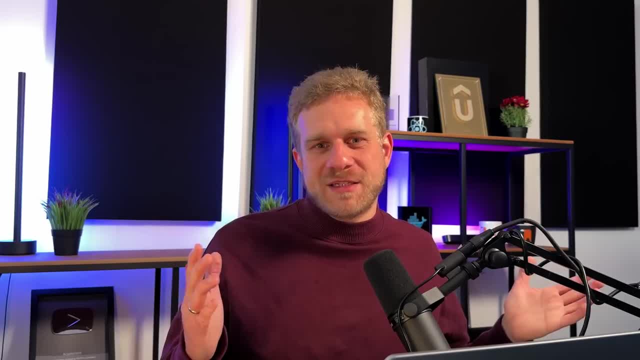 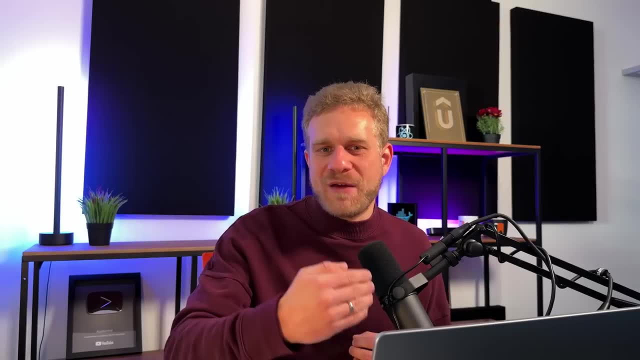 is only going to accelerate. So, therefore, what's the next phase? Or is this the last phase? Well, things will continue to change. The next phase is going to be the last phase of the next phase, But I think we have reached an important point in the history of javascript frameworks, and 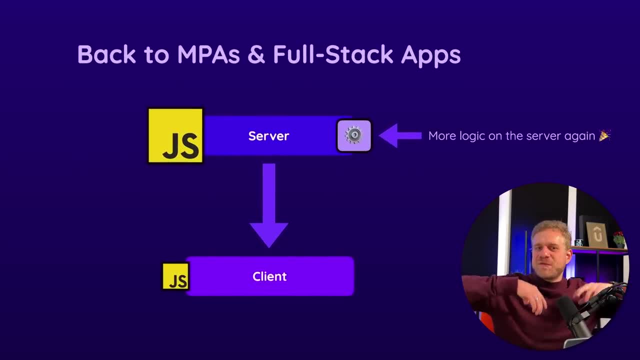 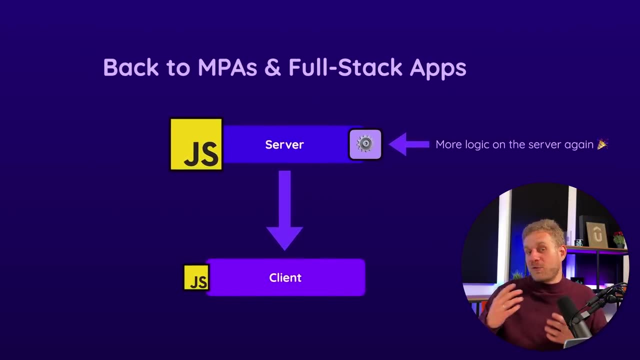 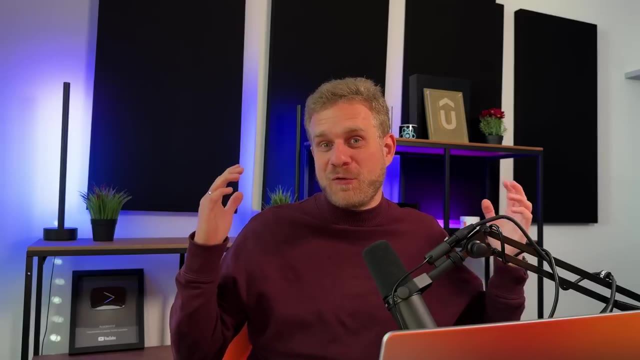 javascript development. I think, as mentioned, that this full stack approach, which combines these best aspects of the different ends, is the future, But of course we'll see which new tools and technologies we will gain to make all these parts even more fun and easier, And therefore, of course, you could almost say that we're back at the point. 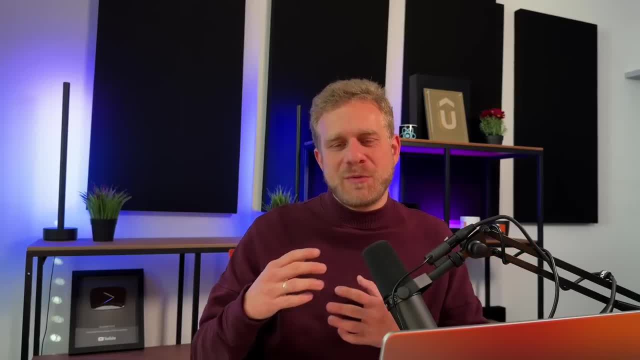 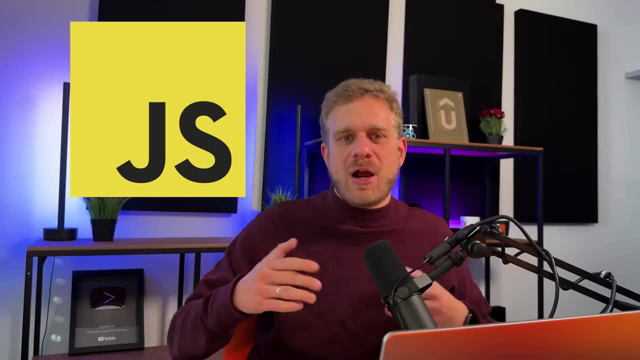 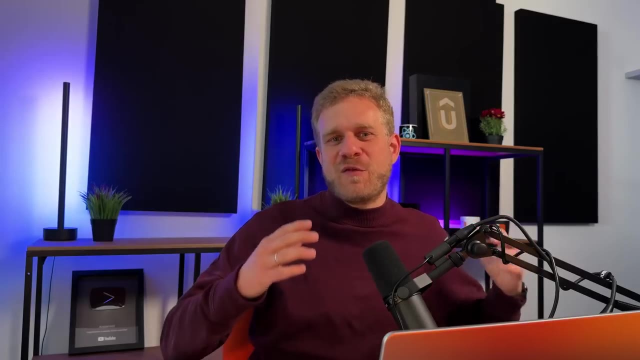 where we started. We are not back in the legacy javascript world, but we are back in the multi-page application world. just that: we used PHP in the past and now we use javascript. But the important difference is that we now do have the best of both worlds. We now do have modern javascript with 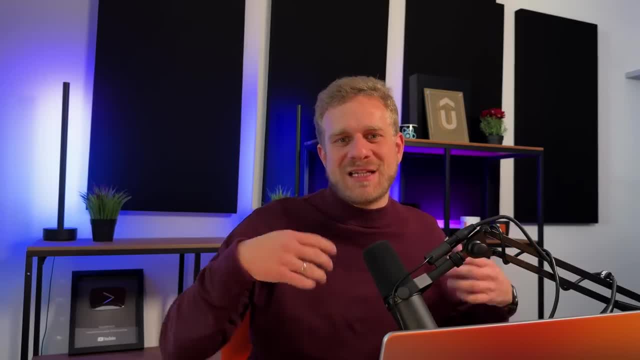 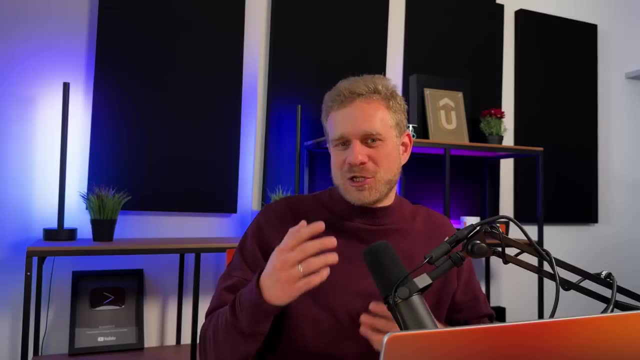 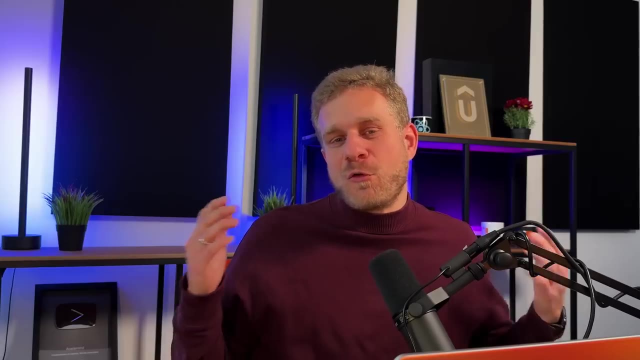 modern features combined with the very powerful frameworks like React or Angular that make building highly interactive web user interfaces a breeze and much easier than it used to be. But it is now moving into a direction where we ultimately start combining that with more backend capabilities again, And of course, it's not guaranteed that it will always be React and Next It might be analog.